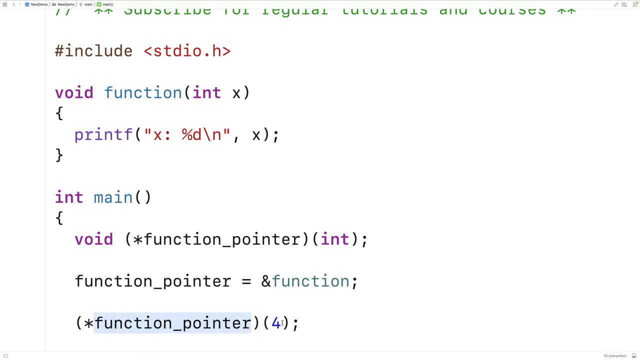 pointer and we're accessing the function and we're calling it with the argument four And if we save and run this, we should get x, colon four, as output. So we can also have pointers to functions that return a value. So for example we could say here: double add, double x, double y and the add. 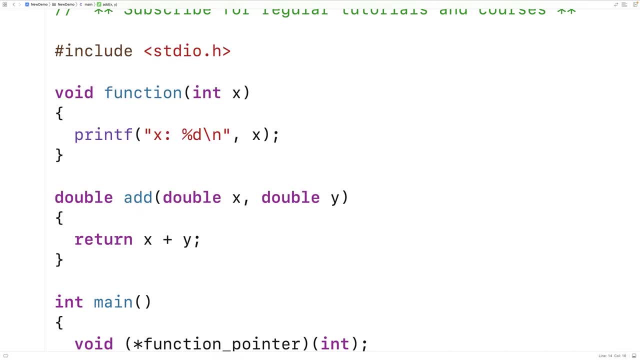 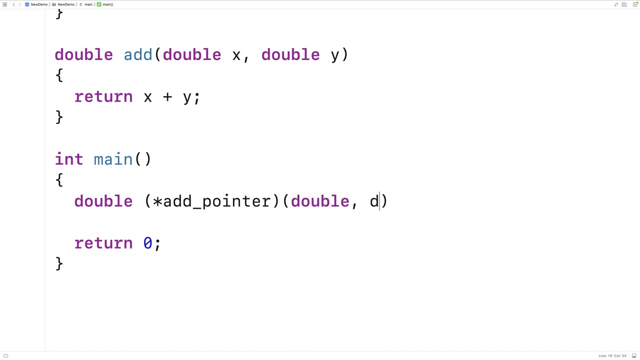 function is going to return x plus y, And then down here we can make a pointer to this: add function. So here we'll say double star, add pointer, and then double, comma, double. So this here would declare a variable called add pointer. It's going to be a pointer to a function. 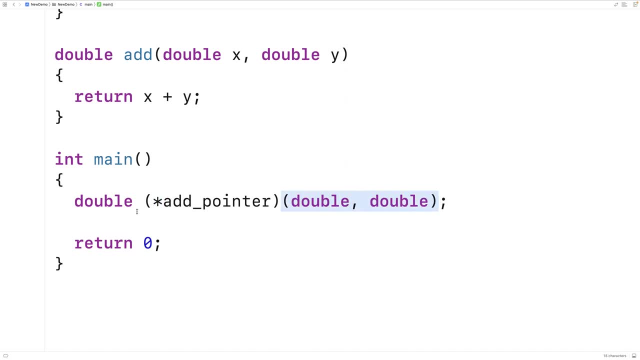 that accepts two double arguments and returns a double value. We could assign the function memory address right here, and I could say and add. I could also just say add, though I don't actually need the and, and this will work okay. We could call the function two. So here we'll say: double a is equal to 20.. Double b is equal to 30.. 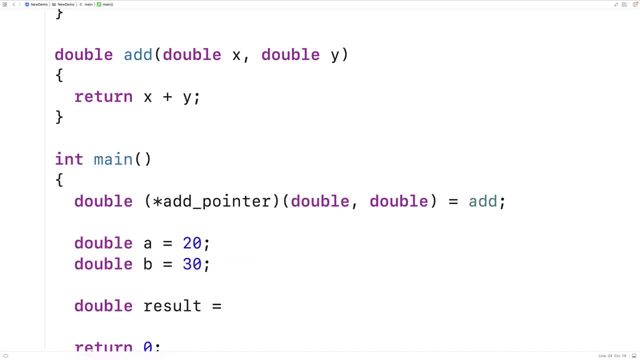 And we'll say: double result is equal to. and we'll call a function like this. We'll say: add pointer a, b And this is actually okay. There's no need to dereference the pointer- And we'll print out the result to verify that everything went okay. 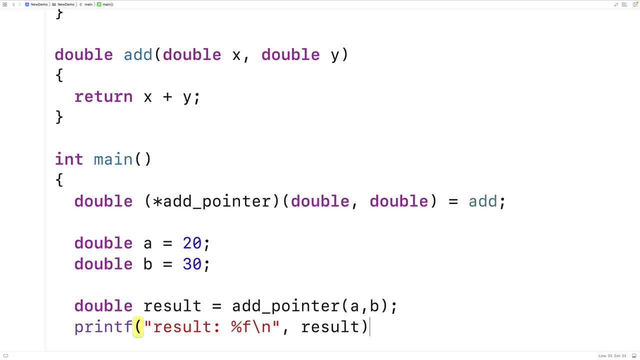 F backslash n for new line And we'll put the result here. And if we save around this, we should get a result of 50. And we do. We can also have arrays of pointers to functions. To do this, we'll make multiple functions that have the same return values and the same number and types of parameters. 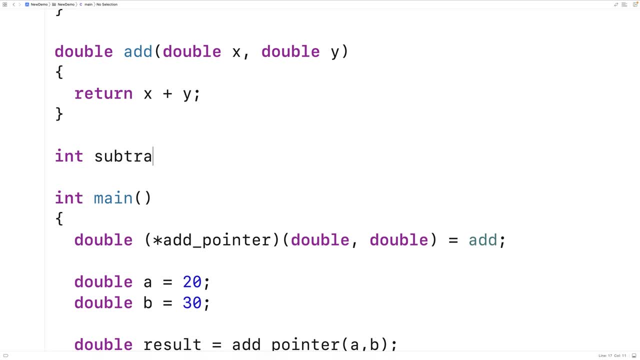 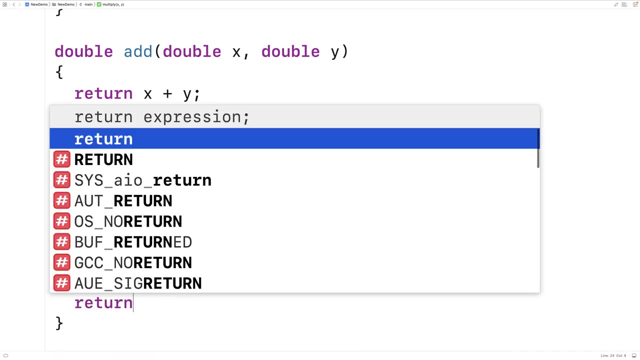 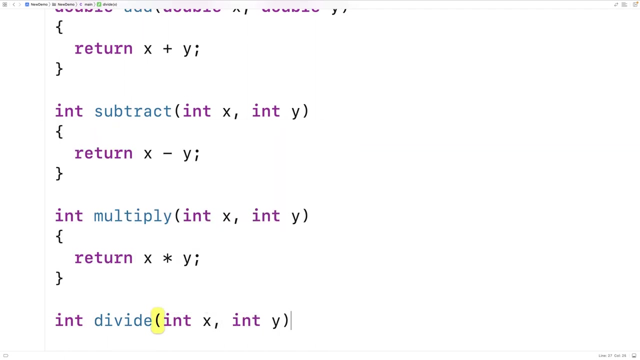 So we'll say int subtract int x Int y, And this function will return x minus y. We'll say int multiply Int x Int y, And this function will return x times y. And then we'll say int divide Int x Int y, And this function will 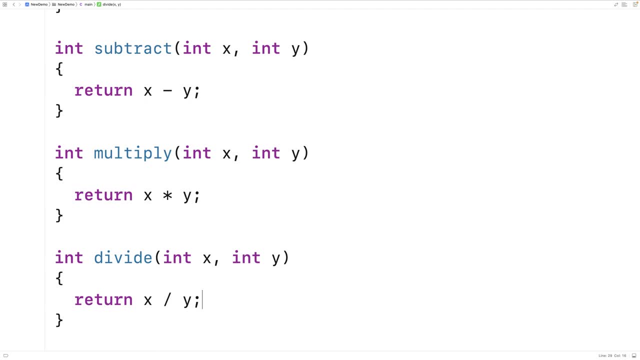 return x divided by y. We can make an array of pointers to these functions. So down here in the main function We'll say int- star array, open bracket, close bracket, And then we'll have int, int. And this is declaring an array of pointers to functions that accept two int arguments. and 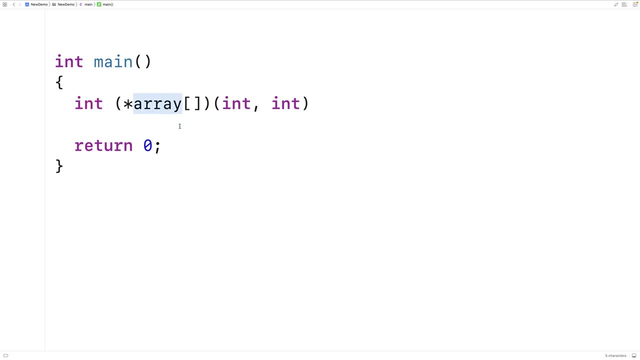 return an int value And it's going to be called array. We can initialize the function. We can initialize the function. We can initialize the function. We can initialize the array right here. We'll say is equal to open squiggly bracket And we'll put in our function. 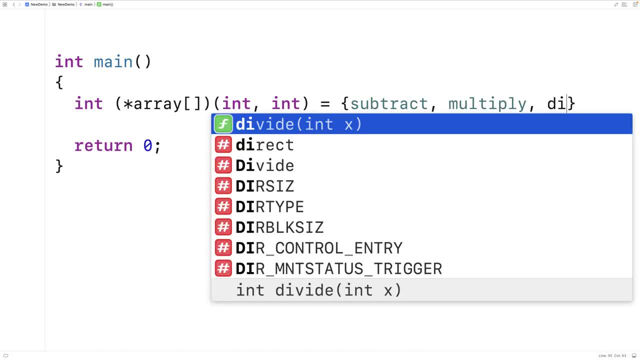 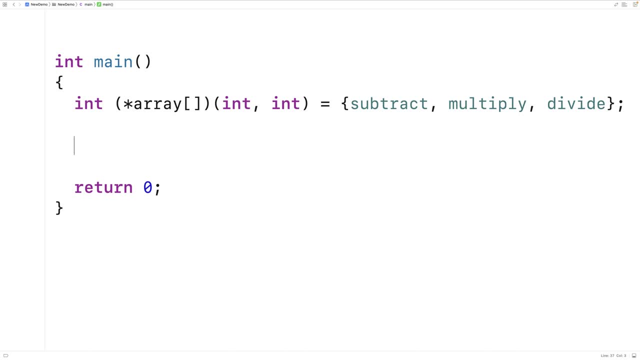 names. So subtract, multiply and divide. Now we can call these functions using this array. So I could say int product is equal to star array at index 1, 3, and 15.. And then we'll try to output the product. 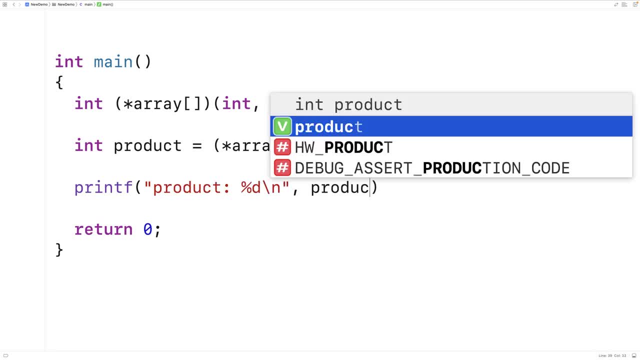 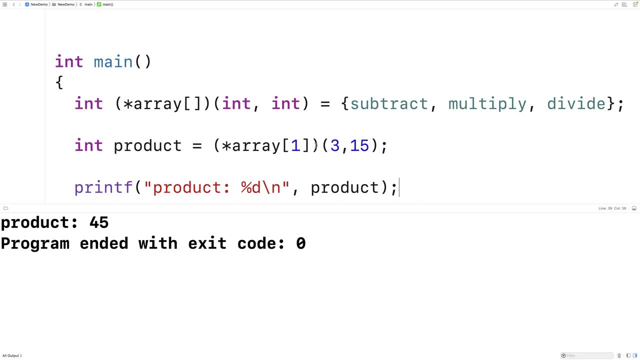 So we'll say product And then we'll put product here And if we save this and run it, we should get product 45. And we do, And that's because array at index 1 is a pointer to that multiply function. 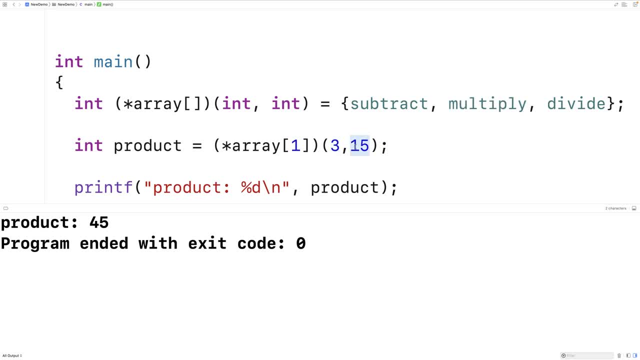 That's going to multiply the arguments 3 and 15.. And we get back the return value 45 that we stored in product there. Now two of the more useful things we can do with pointers to functions is create functions that themselves return a pointer to a function. Or we can create functions that accept as an argument a pointer to a function. 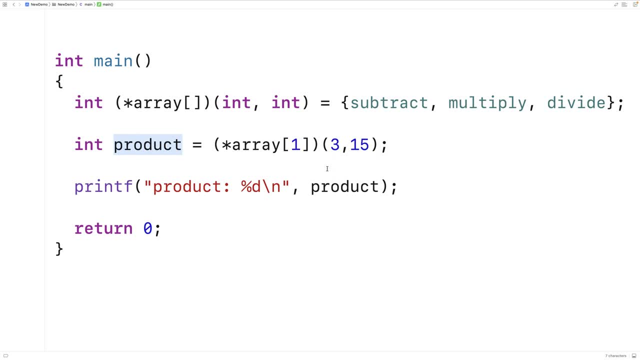 So let's go over examples of both of those ideas. We'll make a function that allows the user to decide between subtracting, multiplying or dividing, And the function will return a pointer to either the subtract, multiply or divide function that we can then use in our main function. 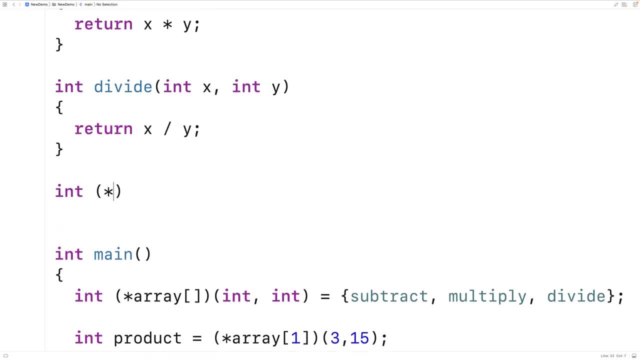 So here we'll say int, star, select operation, which is actually the function itself. That's why we've got open bracket, close bracket there, And then we'll have int and int next. So the syntax here isn't super easy to read. But basically the function is called select operation. 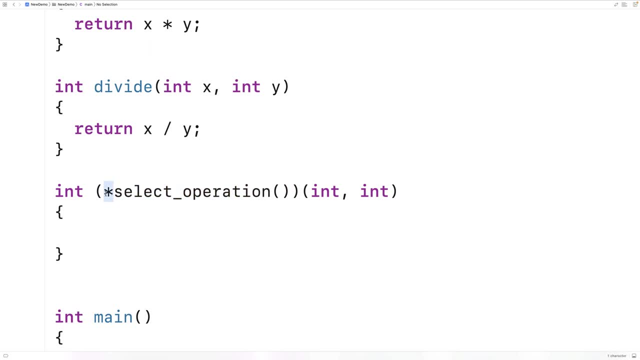 And what it's going to return is a pointer to a function that accepts two int arguments and returns an int value. So next we can actually ask the user for the function that they want to run, the operation they want to use. So we'll say int option is equal to zero. Printf: select an operation backslash n and it'll give them their options. 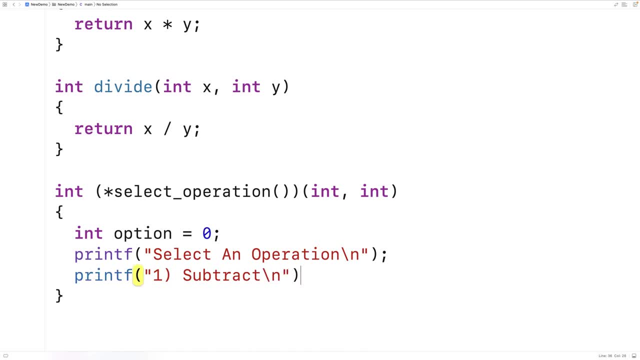 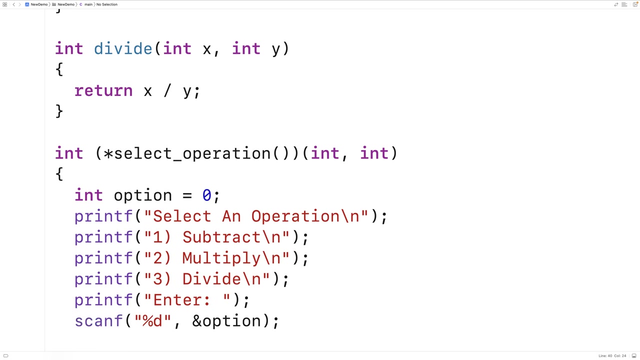 We'll say subtract backslash n, multiply backslash n or divide backslash n, And then we'll prompt the user to enter a choice And we'll use scanf to store the enter into the option int variable there And then we can check the option variable and return a pointer to one of those functions based on that. 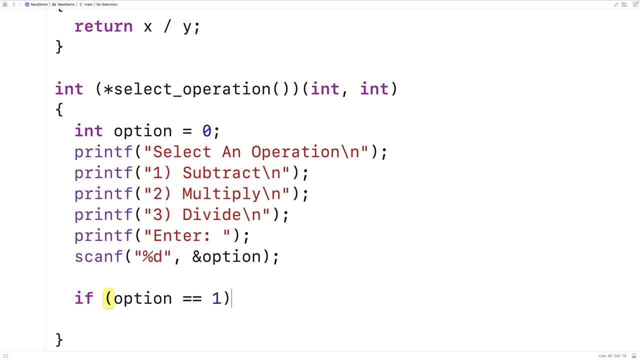 So here we'll say: if option is equal to one, then return a pointer to the subtract function. If the option is equal to two, return a pointer to the multiply function. If the option is equal to three, return a pointer to the divide function. 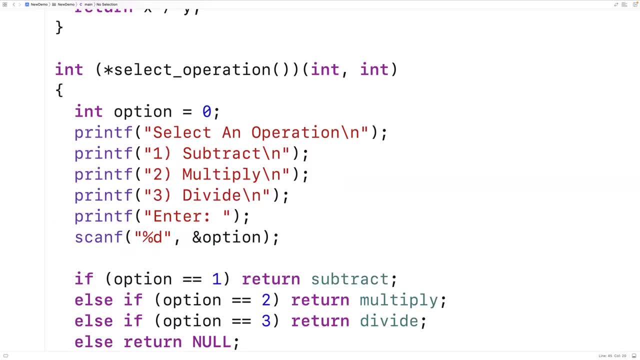 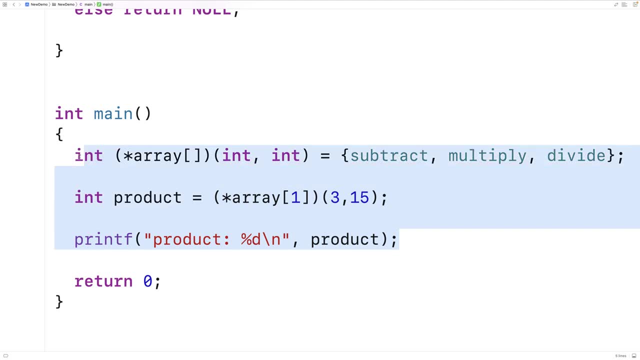 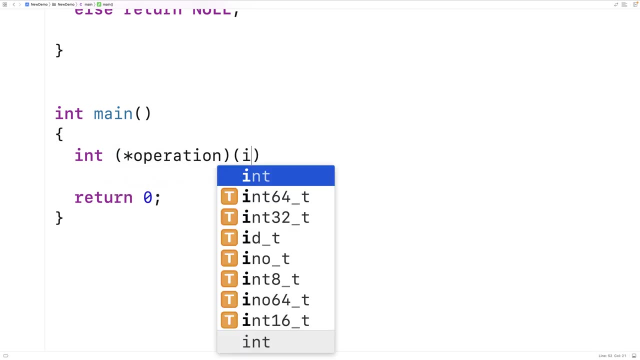 Otherwise we're going to return null in the case of an error. Now we can use this function in our main function. So we'll say here: int star Operation, int, int, And we'll call select operation. So here we're declaring a variable operation that's going to be a pointer to a function that accepts two int values as arguments and returns an int value. 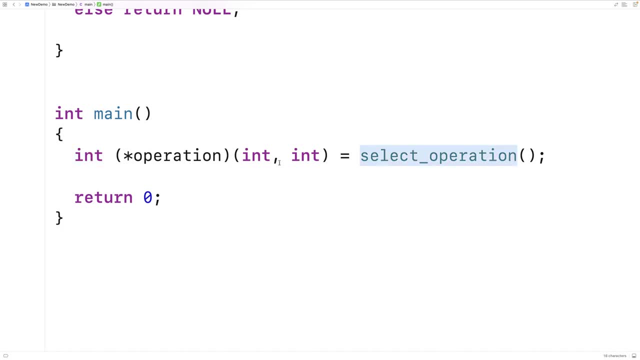 And we're going to assign the result of calling select operation to operation And that's exactly what select operation returns. So next we can call the operation function. We can say: printf answer %d backslash n, and we'll call the operation function now with, say, 20 and 5.. 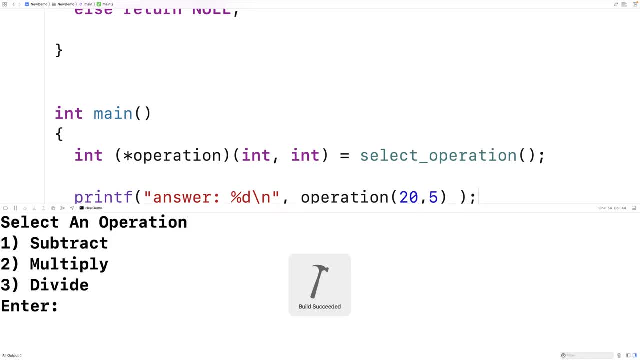 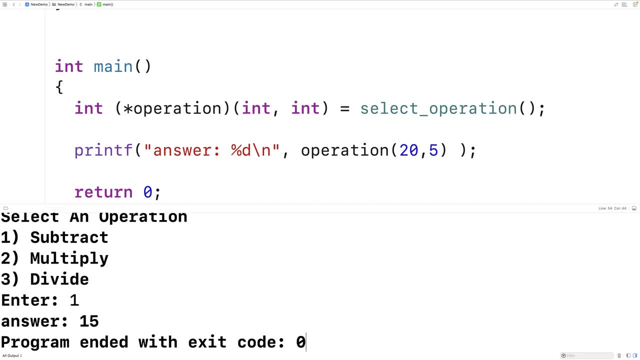 So we can save and run this. And if we select the subtract operation with 20 and 5, we'll get an answer of 15.. If we select multiply, we'll get an answer of 15.. If we divide, we get an answer of 100. 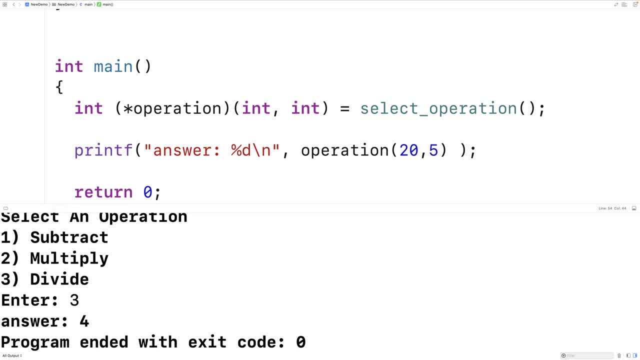 If we select divide, we get an answer of 4.. So that's how we can return a pointer to a function in C, And that's one useful application of pointers to functions. Now let's try creating a function that accepts a function pointer as an argument. 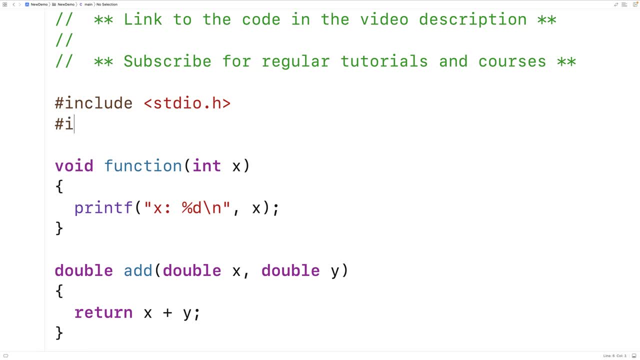 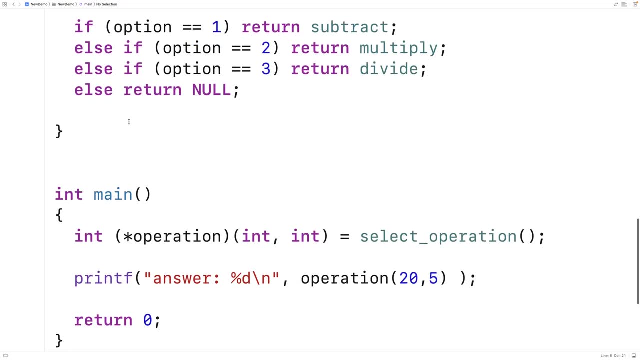 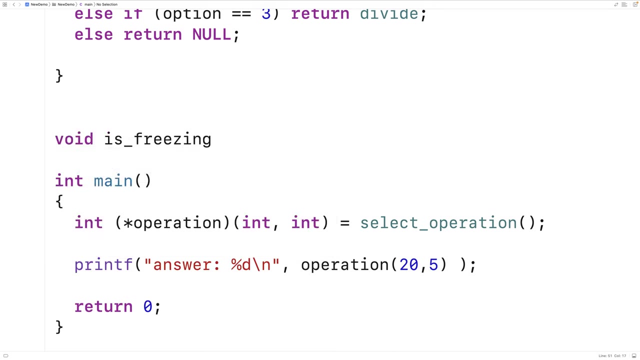 We'll actually include the std boolh library just so we can use the bool type And true and false values. And then down here we'll make a function called isFreezing And the goal of this function is to check whether it's freezing or not. 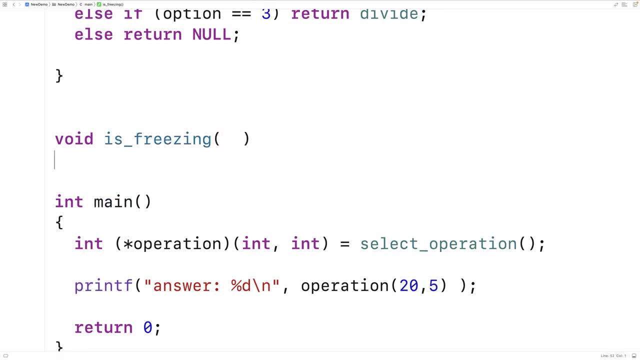 But we don't know whether it's Celsius or Fahrenheit that's being used as a unit for the temperature. So as an argument, the function is going to accept a pointer to a function. We'll call the parameter freezeCheck And we'll have int here. 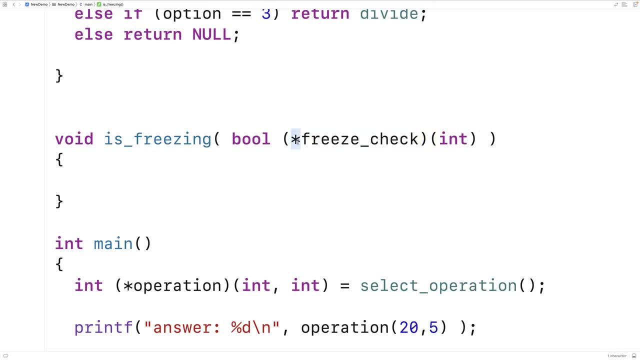 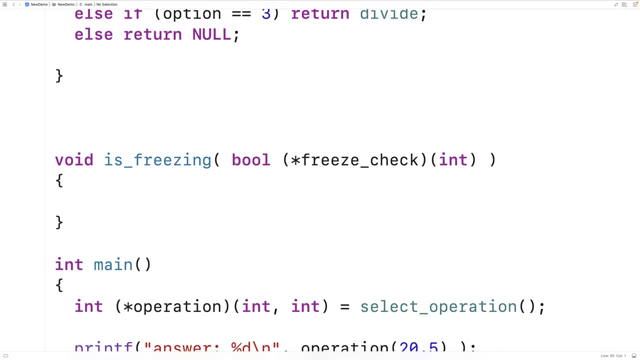 But the parameter freezeCheck is a pointer to a function that accepts an int as an argument and returns true or false, a bool value. We can then make multiple functions to check the temperature to see if it's freezing or not. So we'll say bool: freeze. underscore C. 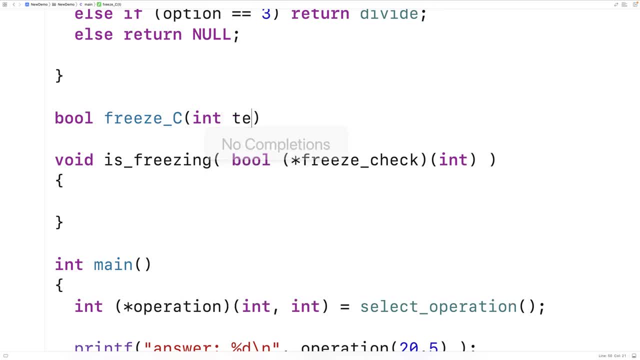 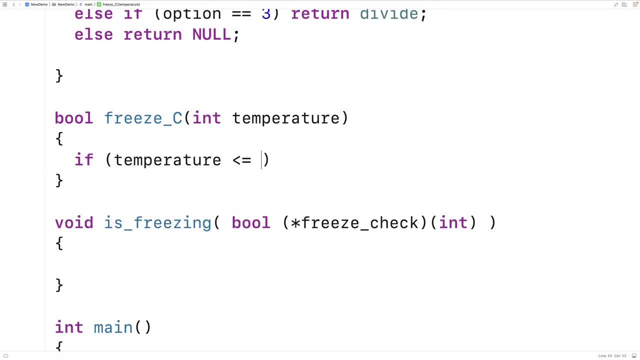 And this is going to check to see if it's freezing or not, And this is going to check to see if it's freezing in Celsius. So we'll say int temperature And if the temperature is less than or equal to zero, we're going to return true. 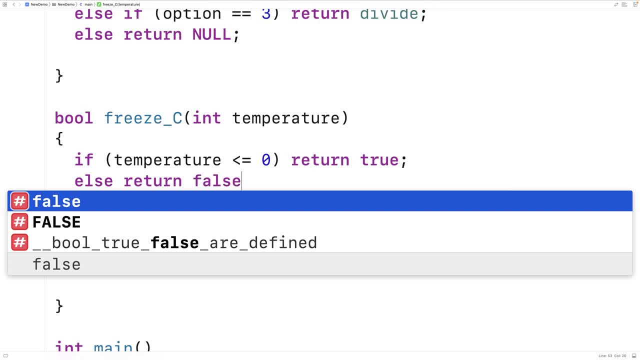 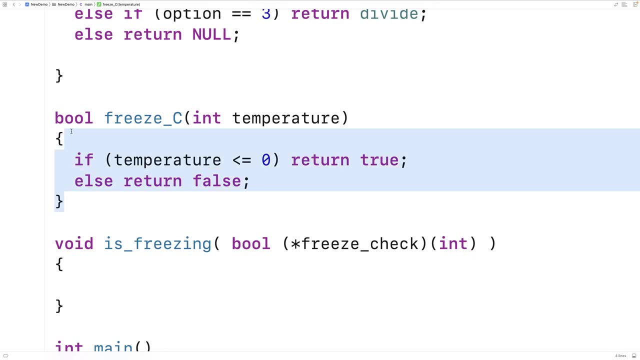 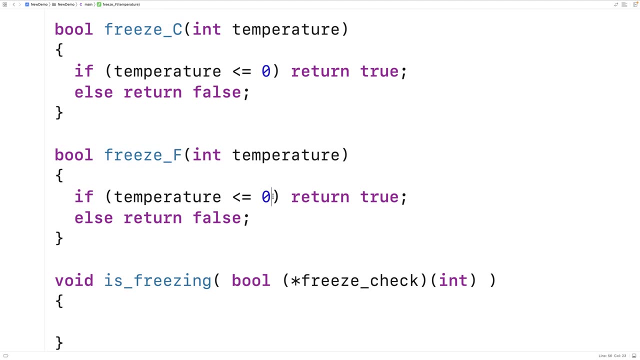 Otherwise we're going to return false. So freeze underscore C is going to check to see if it's freezing in Celsius. We'll make a freeze underscore F function to check to see if it's freezing in Fahrenheit. So at Fahrenheit it's going to be when the temperature is less than or equal to 32.. 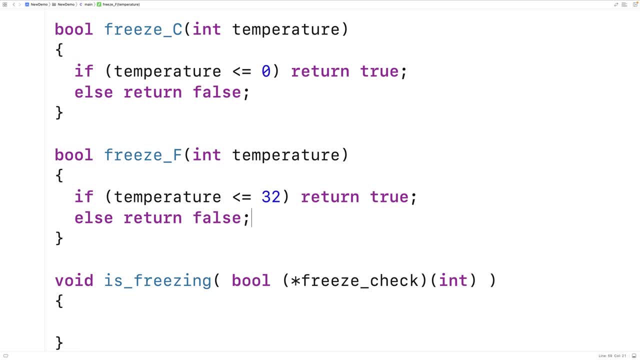 So now we can pass to is freezing either a pointer to freeze underscore C or a pointer to freeze underscore F, And we can change the behavior of is freezing by virtue of the function we've passed into it. It'll either check whether it's freezing in Celsius or Fahrenheit, depending on the function. 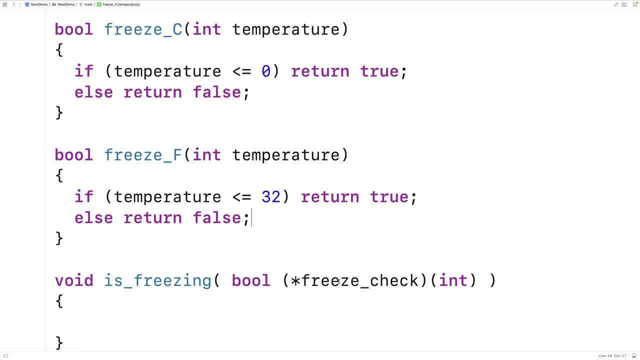 We call this type of function a callback function. We call this type of function a callback function. It's a function that's going to be called back later by this function here. It's going to be used at some later point in the body of this function to do some work. 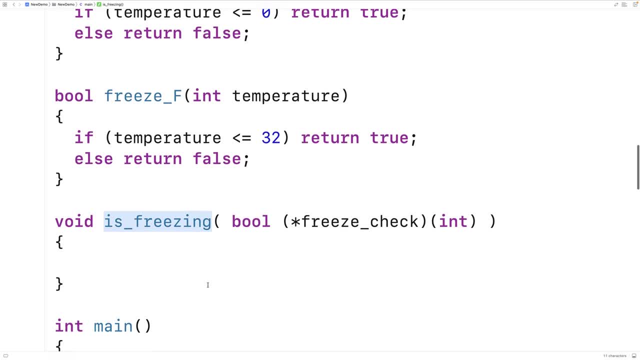 Next let's implement the is freezing function itself. So we'll say: int. temperature is equal to zero And it will prompt the user to enter the temperature And we're going to let them know whether it's freezing or not. So we'll say printf- enter temperature. 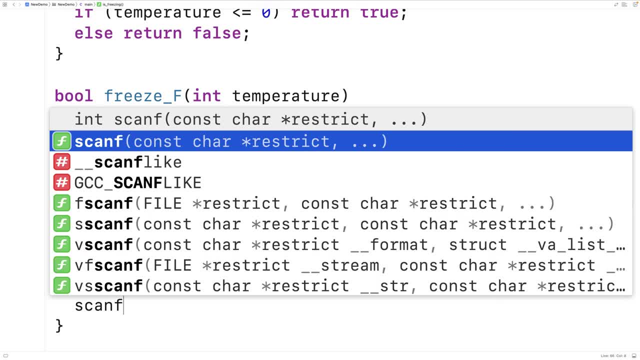 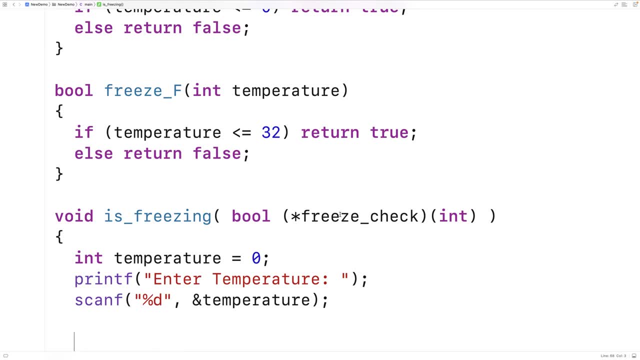 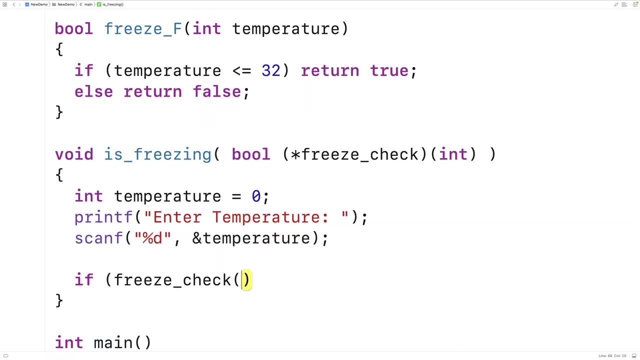 And then we'll store the enter into the temperature variable And then we'll use the freeze check function to check whether it's freezing or not. So we'll say: if freeze check with this temperature as an argument returns true, then printf it's freezing. backslash n. 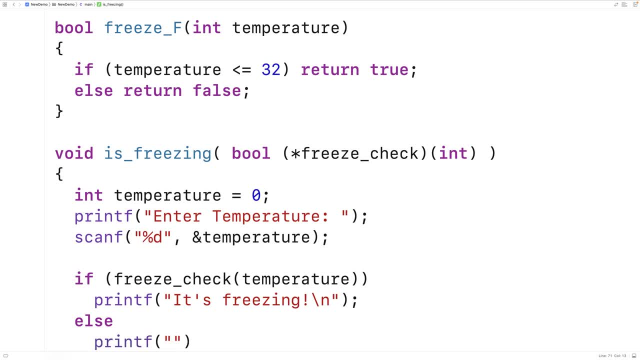 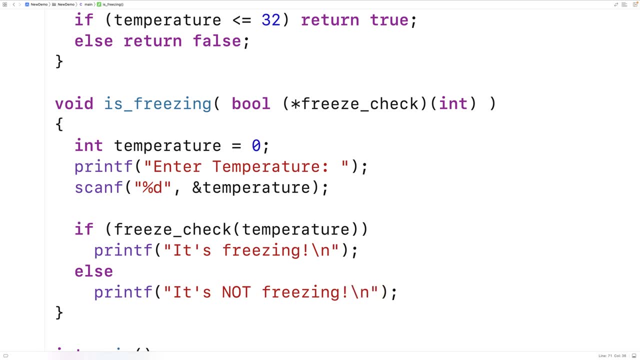 Otherwise printf that it's not freezing. So we'll say it's not freezing. backslash n. And again, the important part is that this function here freeze check- is going to be different depending on which argument was provided to is freezing. 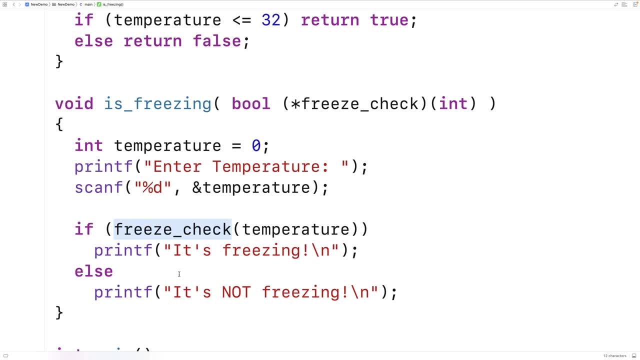 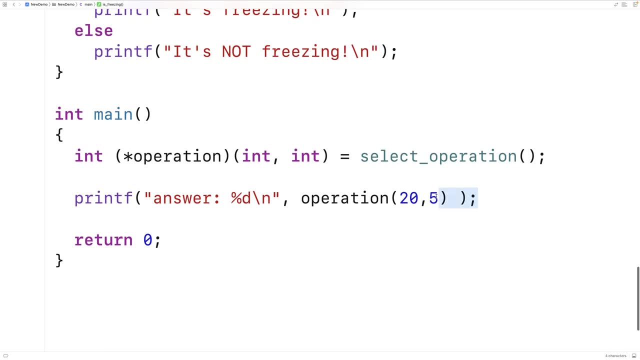 We could be checking in Fahrenheit or we could be checking in Celsius. We're leaving it to this callback function to determine that. Let's try out: is freezing now? First we'll try it out with Celsius, So we'll say: Celsius, throw in some new lines, and then we'll say: is freezing? 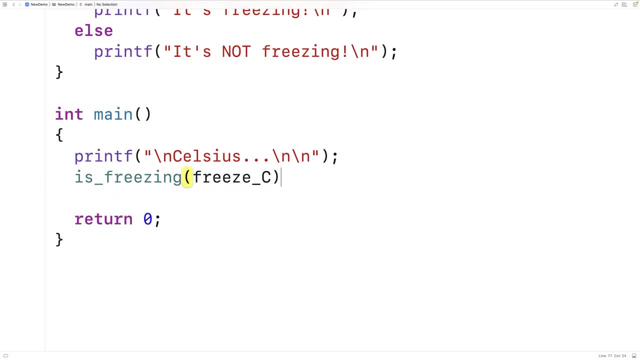 And we'll call it with freeze underscore C And then we'll say: is freezing freeze underscore C? So we save this and run it. It says: enter temperature: If we put a negative 5, we get it's freezing. If we say 5, we get, it's not freezing. 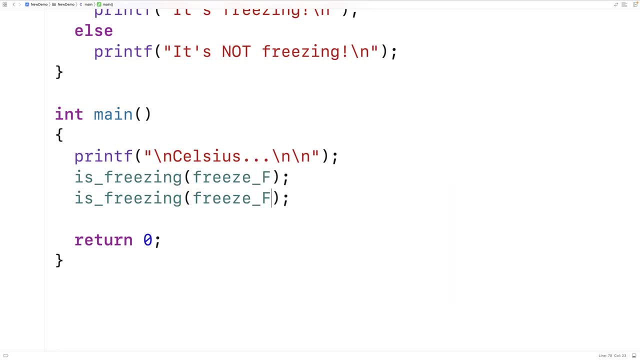 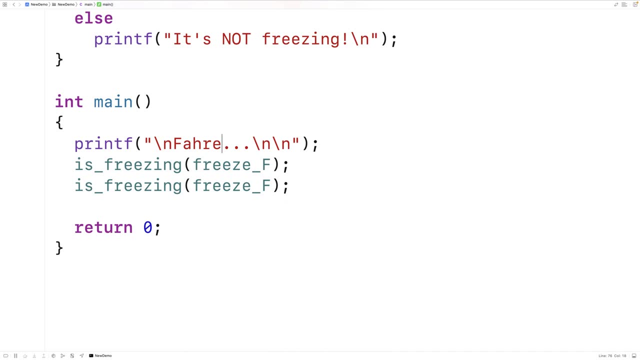 If we try it now with freeze underscore F and we'll say Fahrenheit here now instead So Fahrenheit, And we save and run it Now, if I try negative 5, we get it's freezing. If I try 5, we also get it's freezing. 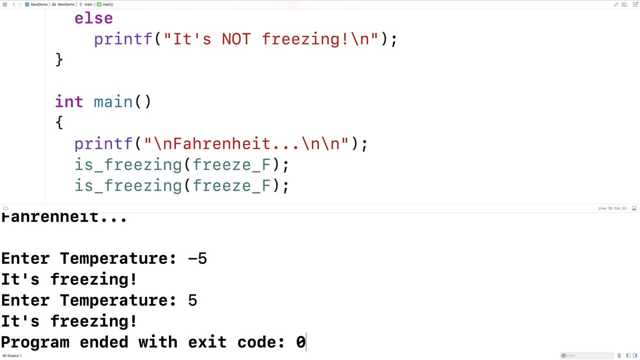 So we're getting a different result from the is freezing function, And the reason why we're getting that different result is because we're passing in a different callback function, a different pointer to a different function. So this ability to pass a pointer to a function as an argument to another function. 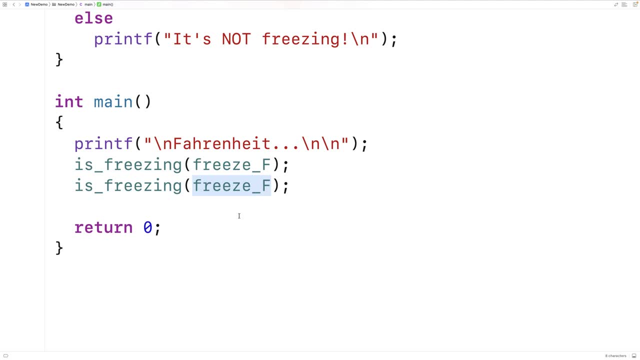 is really important in programming in general. For example, even the built-in quick sort function It comes with the C standard library Depends on this. We actually provide a pointer to a function as an argument to quick sort to help carry out its work. 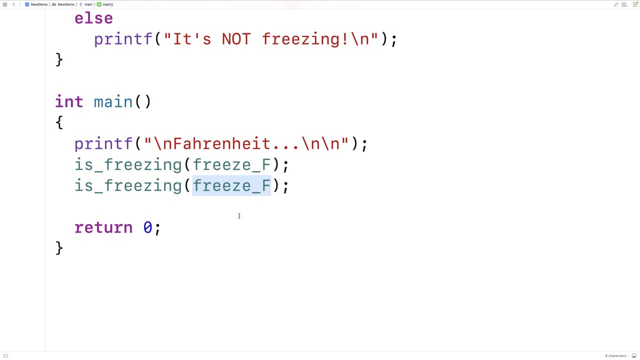 Now, with function pointers we don't allocate space. So with regular pointers we might allocate space for dynamically allocated memory on the heap using functions like malloc, calloc, and then free to free the dynamically allocated memory. With function pointers we don't do that. 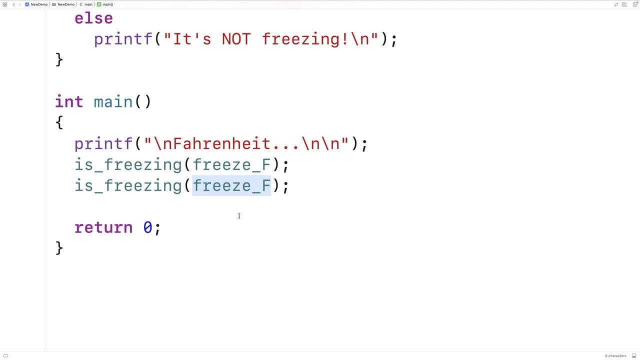 Function pointers are pointers to instructions. They're not pointers to data. They're really a different kind of thing. We also don't do pointer arithmetic with function pointers. If we try that, we're going to have a bad time. I'll just show you what I mean here. 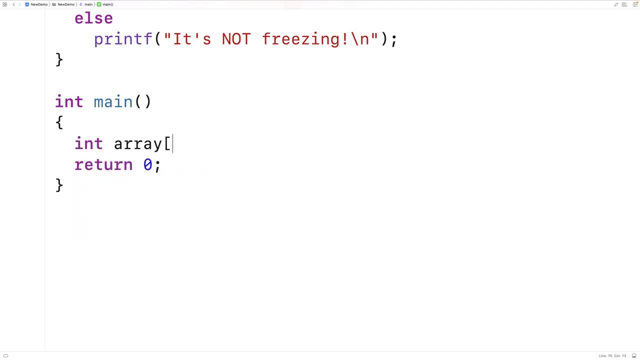 With a regular pointer. let's say we've got an array here with 5 values in it: 1, 2, 3, 4, 5. We can make a pointer here. We'll say int star pointer. So pointer is equal to end array at index 2.. 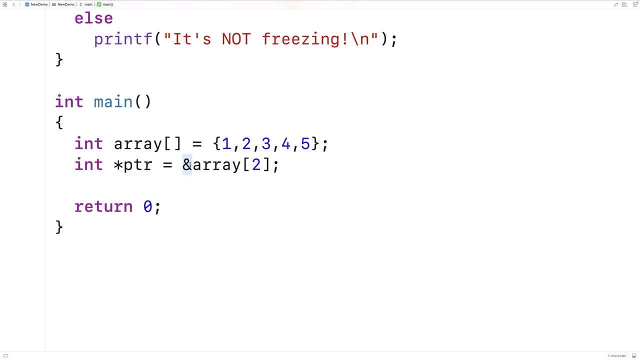 So pointer is storing the memory address of the array at index 2, which is going to be that index there, So it's going to have a pointer to that value 3.. We can use pointer arithmetic So I could say pointer plus plus.